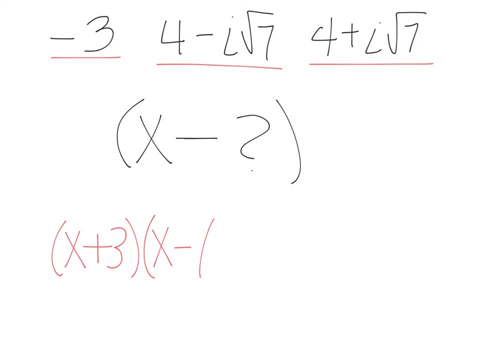 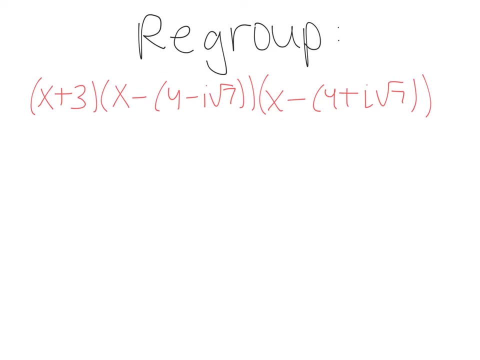 3.. Then x minus 4 minus i root 7.. And x minus 4 plus i root 7.. Now we will regroup, Leaving the x plus 3 as it is. we'll distribute the negative, So write: x minus 4 plus i root 7, and x minus 4 minus i root. 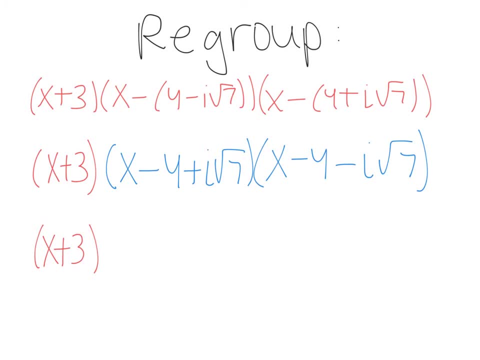 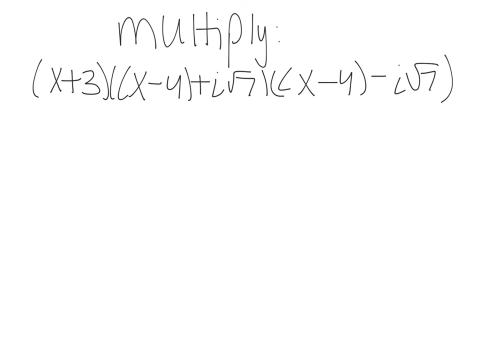 7. Now regroup so that the x minus 4's are together Like this: And x minus 4 minus i root 7.. So we didn't change anything, but we did put the x minus 4's together. so you can visualize that Now we will multiply these. 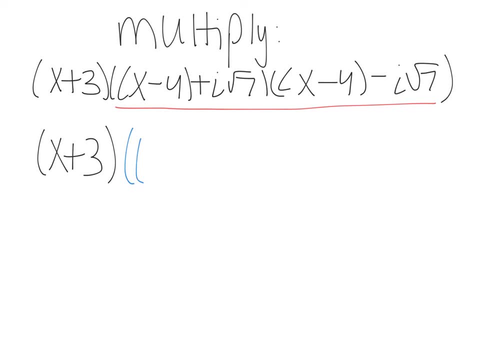 two. So that will be x minus 4 squared, because we multiplied these two together and we'll multiply these two together And since it's plus minus, you know that then you'll just need to multiply these two together. So that's x minus 4 squared, minus 7, i squared, i squared. 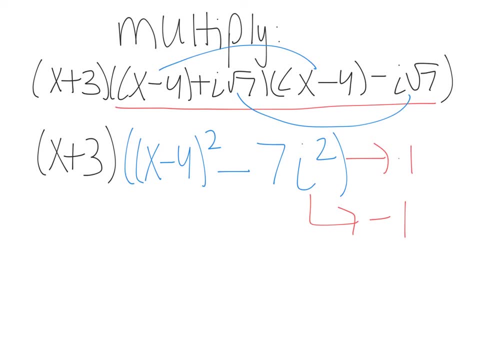 is the same as negative 1,, so this would be plus 7.. Continue to multiply, So that would be x squared minus 8x plus 16.. And don't forget the 7., Which will make this 23.. Now we can multiply these two together. 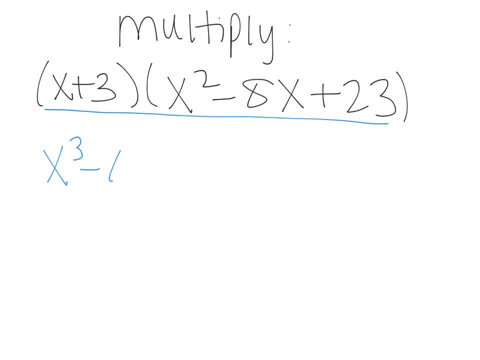 So first distribute the x, So x cubed minus 8x squared plus 23x, Then the 3. Plus 3x squared minus 24x plus 69. Then combine all of these terms, So x cubed minus 5x squared minus x plus 69. So now we